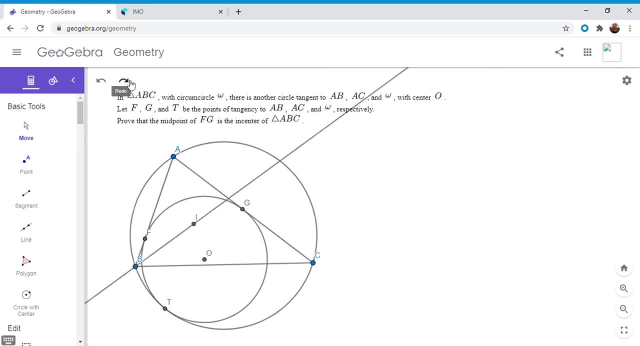 And I'm going to tell you why I'm doing this. First of all, it's convenient to do it in general Because the angle bisector of angle B always meets the arc AC at the midpoint, So D is the midpoint of arc AC. 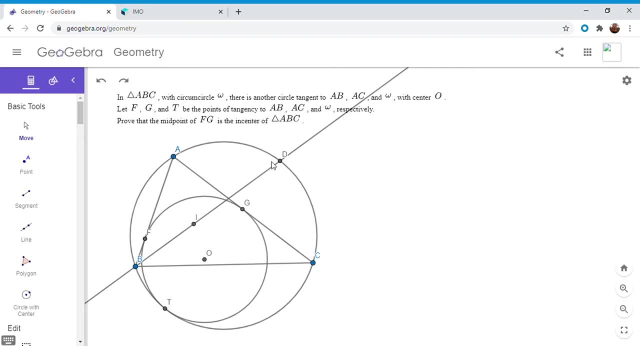 I've mentioned that many times on my channel- And that's because equal angles intercept equal arcs. And then we can do the same with extending CI to meet the circumcircle of E, And so D is the midpoint of arc AC and E is the midpoint of arc AB. 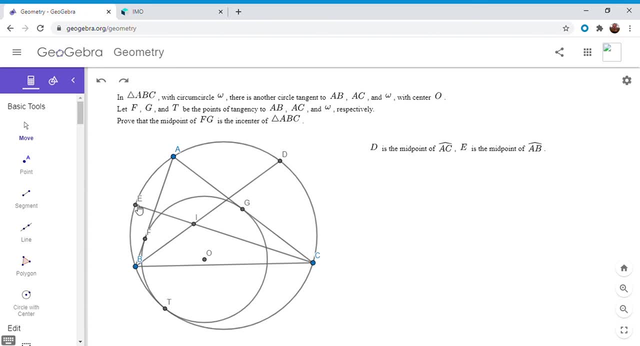 Now, why did I do this? Well, the midpoint of an arc has a special property: that when you draw the tangent to it, that tangent line is parallel to the chord between the two endpoints of the arc. So basically, the tangent at E to omega is parallel to AB. 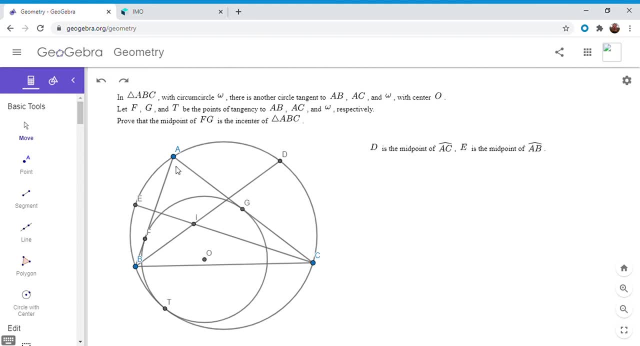 And the tangent at D similarly is parallel to AC, And so that will come in handy later. So some people are familiar with homothetes, So maybe a kind of advanced concept. But they'll recognize that if, since omega and the mix, the linear in the circle, are both tangent at T. 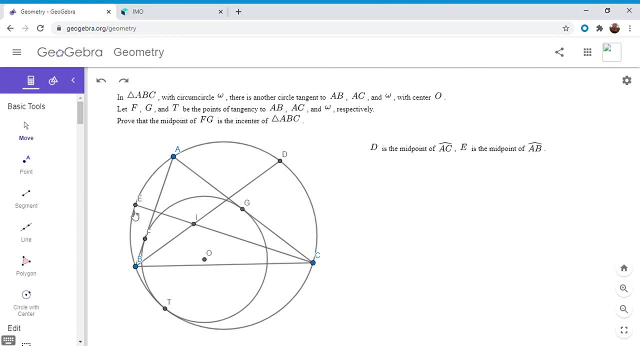 if the tangents at F and E to the two circles are parallel, then they'll see immediately that E is parallel to the two circles. Then they'll see immediately that E is parallel to the two circles. Then they'll see immediately that E is parallel to the two circles. 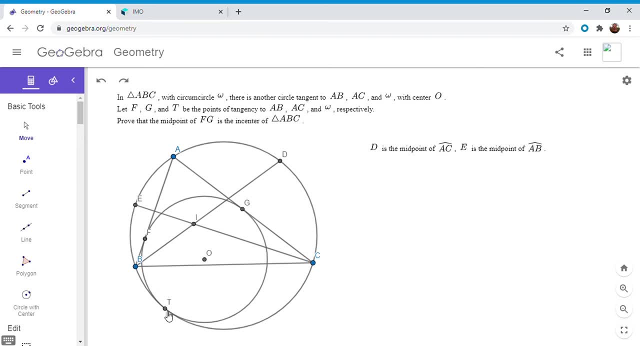 Then they'll see immediately that F and T are collinear. But I don't think it's that obvious, So I'm going to go prove it out here. Okay, So, like I said, the tangent to the circle O through point E is parallel to AB. 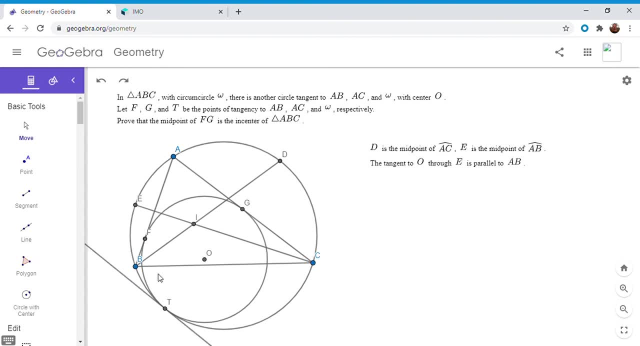 So I'm going to draw that tangent And I'm also going to draw the tangent to both of these two circles through T, Okay, And I'm going to let those meet at point H. And then what I'm also going to do is I'm going to extend line AB to meet the tangent through T at a point J. 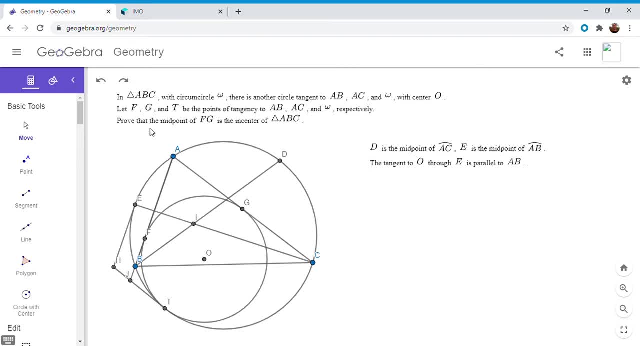 So why am I doing this? So I want to leverage the fact that AB is parallel to this tangent at E. So that's one reason why, And also we have lots of tangents to circle, So we have a tangent to circle. 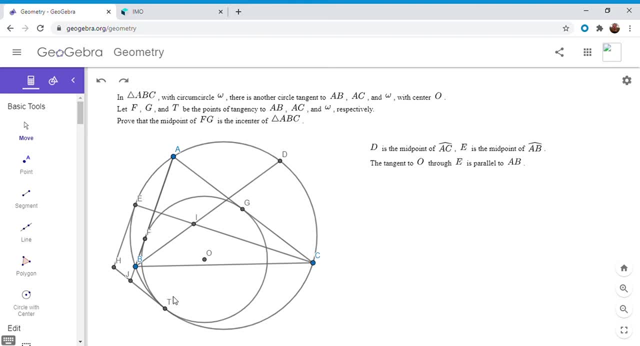 So we have a tangent to circle omega at E, We have a tangent at F And we have a tangent at T, And intersection points of any two tangents are equidistant to both circles. So I'm going to try to leverage that fact here. 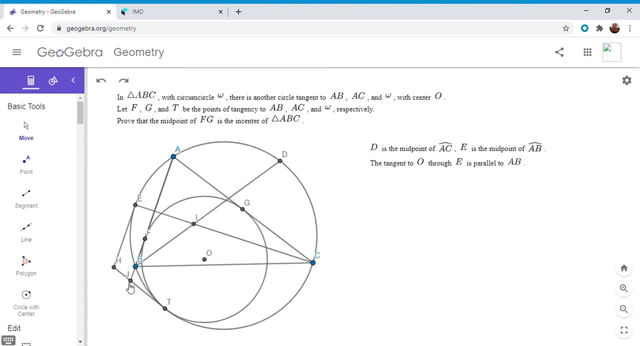 And that's kind of why I got them all to intersect. So ultimately, I want to show that E, F and T are collinear. Okay, But since the tangents to the two, tangents from any point to a circle, are equal, 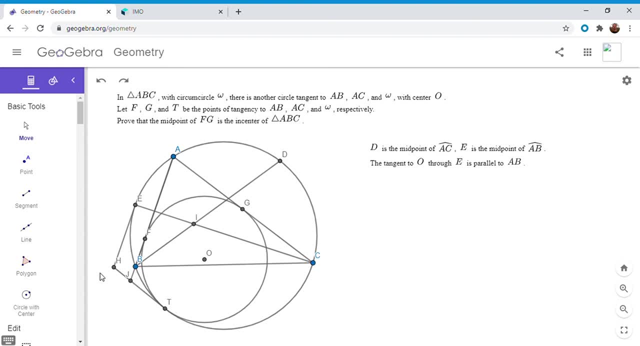 J, T, F is isosceles and E, H, T is isosceles. So showing that those three points are collinear is essentially the same as showing that they're similar isosceles triangles. But that's true because since AB is parallel to the tangent at E, 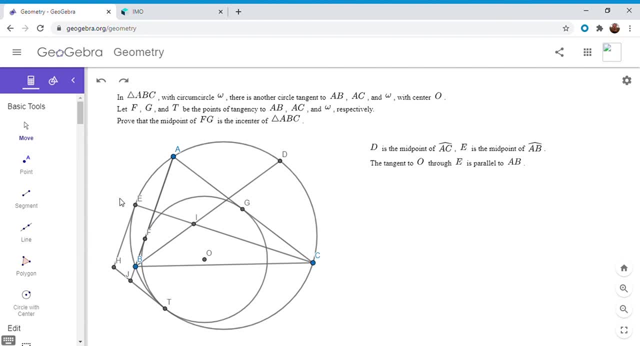 we'd have to have angle T, H. E is equal to angle T, J, F, So those two isosceles triangles would have to be similar, And so E, F, T have to be collinear. So I'm going to write that out a little bit. 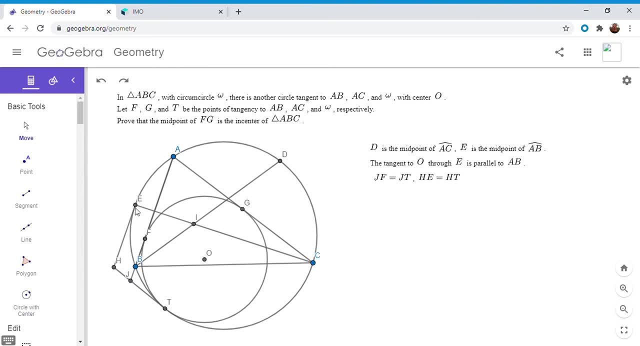 So, like I mentioned, J F is equal to J T, H E is equal to H T, So they're both isosceles triangles. Also, angle T, J F is equal to angle T, H E, because those two lines, A, B and E H, are parallel. 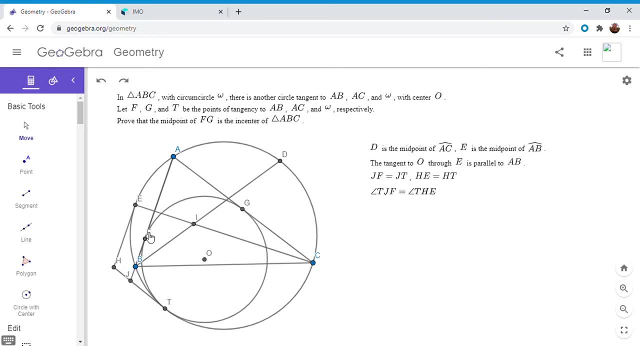 And so if you have two isosceles triangles and not the vertex angle, but two of the base angles are the same, then the two isosceles triangles have to be similar. So T J, F is equal to T H, E. 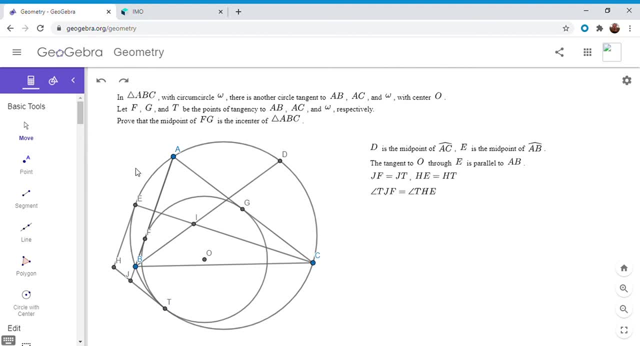 We'd also have to have. J T F is equal to H T E, So I'm going to write that out. So angle J T F is equal to angle H T E, And obviously that means E, F and T have to be collinear. 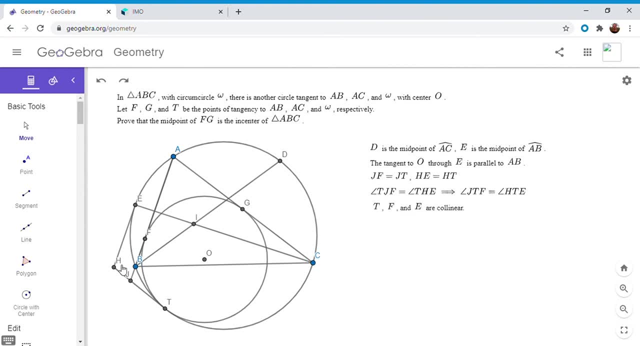 Okay, Um, so I'm going to write that out. So I'm going to write that out, So I'm going to erase some of the work I did to show this and just draw the line through T, F and E. So, like I said, people familiar with homophobes will just recognize that right away. 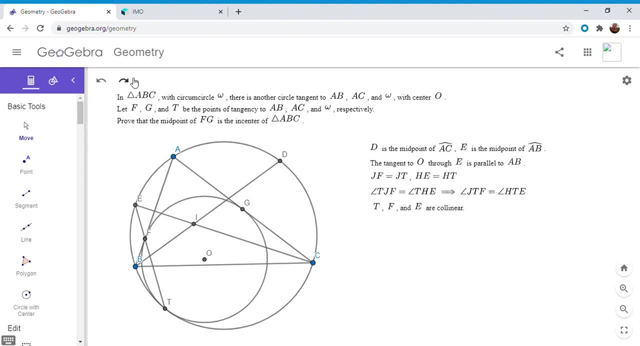 that those three points would have to be collinear And then, by the same logic, T, G and D would also have to be collinear. So I'm going to draw that line And I'm going to move the diagram a little bit, because I don't want it to look like it passes through O. 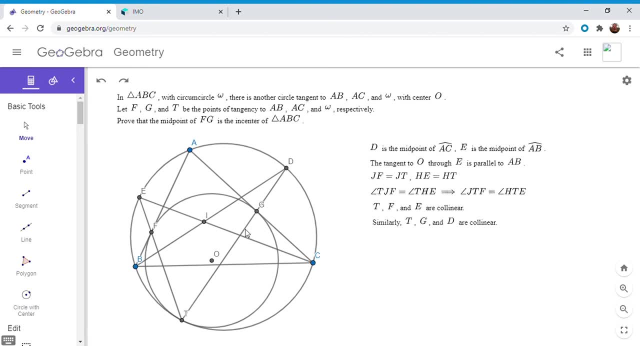 because that's not necessarily true, Okay, Okay. So now this looks like a perfect chance to apply Pascal's theorem, because we have all these points, all these six points intersecting each other, If you take so, if you look at points E, A and D. 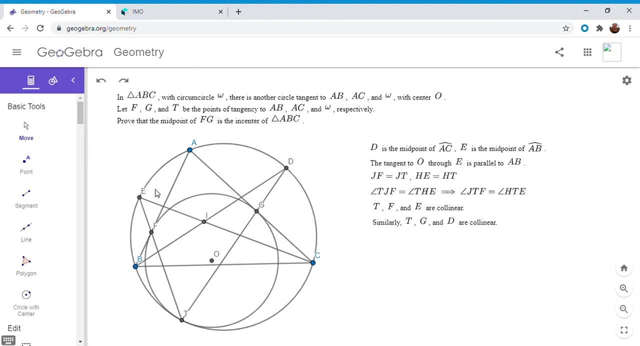 and how they correspond to B, T and C. if you take each point and you connect it to the other two that it doesn't correspond to. so E gets connected to C and T, A gets connected to B and C and D gets connected to B. 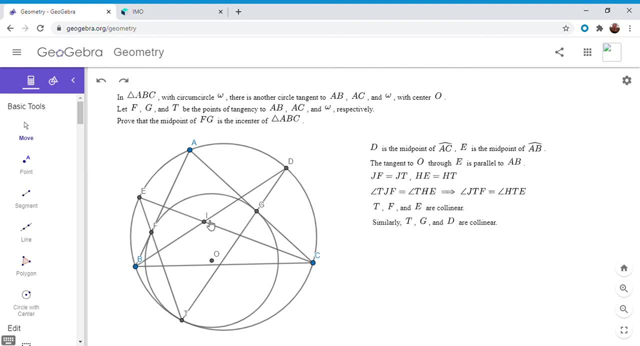 and D gets connected to C and T. and you take the three intersection points F, I and G. by Pascal's theorem they'd all have to be collinear. So F, I and G are those three intersection points and they're collinear. 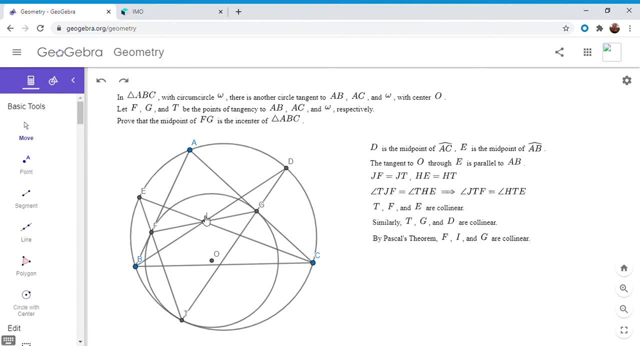 So we're almost there. So we wanted to show that the in-center I is the midpoint of F G. So far we've shown that it lies on F G. So now that we know it lies on F G, how do we know it's the midpoint? 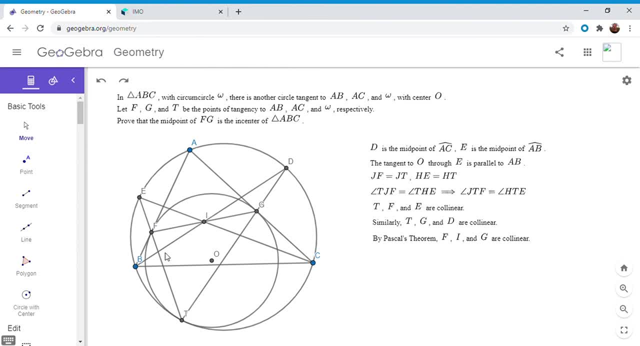 And that's not too hard to see, Because A I is the angle bisector of B A C, So it also has to be the angle bisector of F A G. But if A I is the angle bisector of F A G, 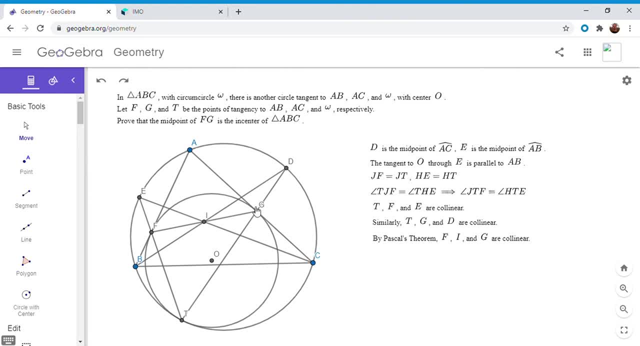 and we also know that the tangents A, F and A G are equal. it's very easy to see from that that F I has to equal I G, And so that proves the problem. Okay, so I just wrote that out here. 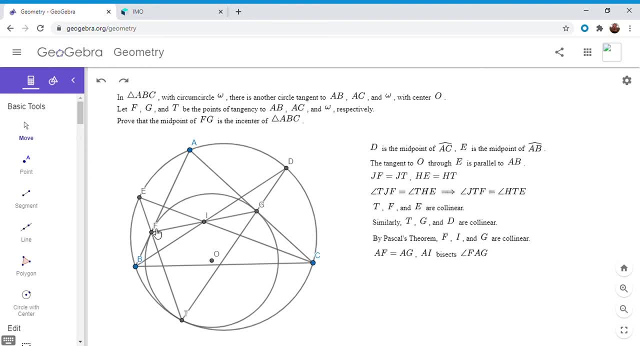 So A F is equal to A G And A I is an angle bisector of F, A G. So because of that in any isosceles triangle the angle bisector from the vertex is also the median. 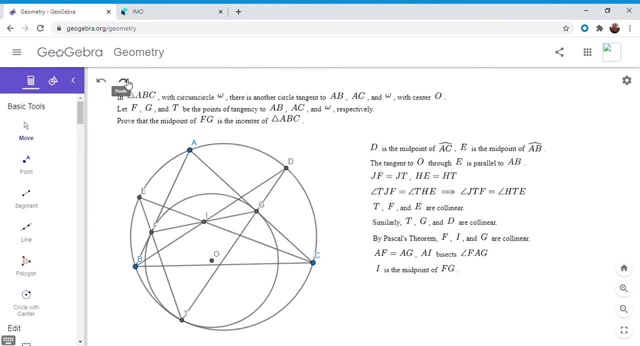 And so we have to have F. I is equal to F G, And so I is the midpoint of F? G, And that solves the problem. So that's part one of this video, A really interesting theorem that I think is also called: 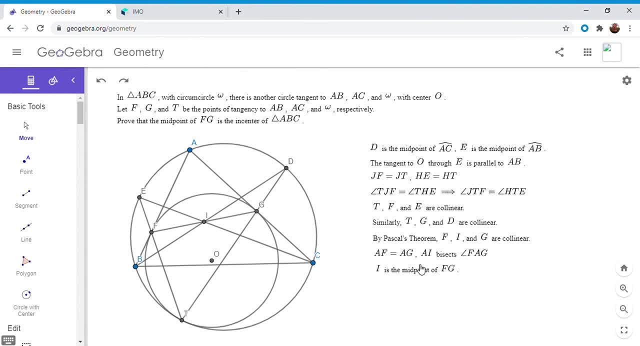 Berry-A's theorem. But now I'm going to try to do a part two. so part two of this video I'm going to show that T I meets the arc B, A, C at its midpoint. All right, So that's a second fact about mixed to linear in circles. 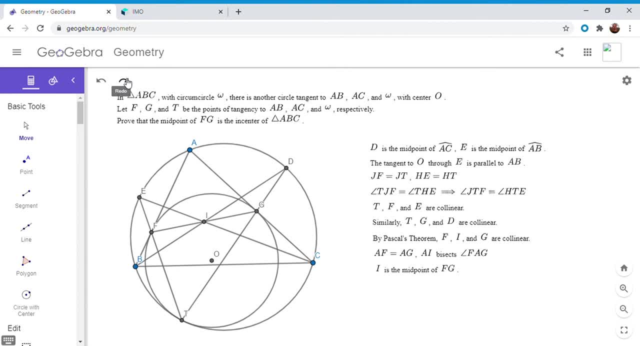 That's very interesting. So I'm going to try to prove that. So I'm going to erase a couple, I'm going to erase the work I did and change the problem statement. So we want to show that T I passes through the midpoint. 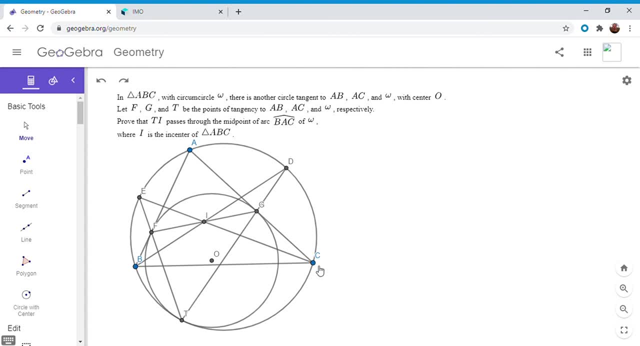 and the arc meets the point of arc B, A, C. How do we do that? All right, So here's where it gets kind of interesting. So if you look at triangle T, F, G, T, I is the median of that triangle. 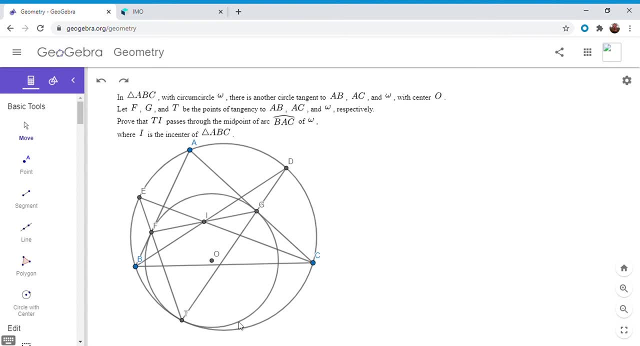 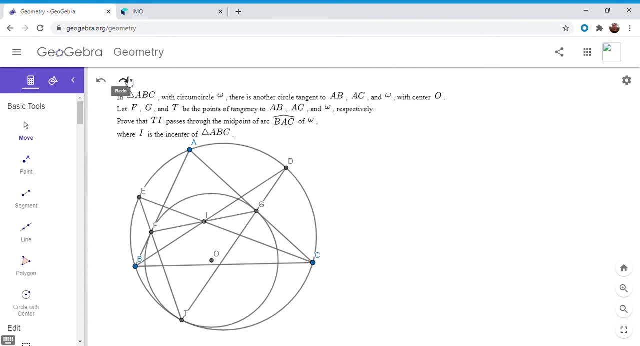 So I'm going to try to prove it, But it comes in handy all the time. I feel like I've used it before on my channel, So maybe some day later I'll create a video on it. But if you have this configuration where triangle T, F, G. 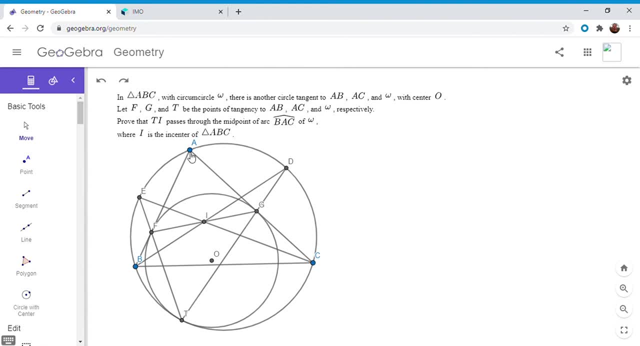 and you take the two tangents at F and G to the circumcircle T, A has to be a submedian from T in the triangle T, F, G. So what does that mean? That means that if you take T, I, which is the median, 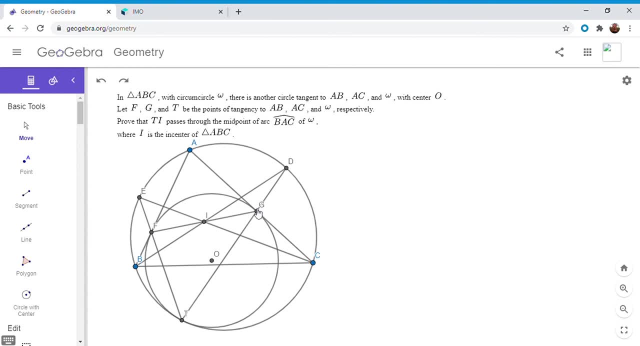 and you reflect it over the angle bisector of F, T, G, then you would get line T A. So I'm going to write some of this out. So first I'm going to let T. I meet the circumcircle at a point. 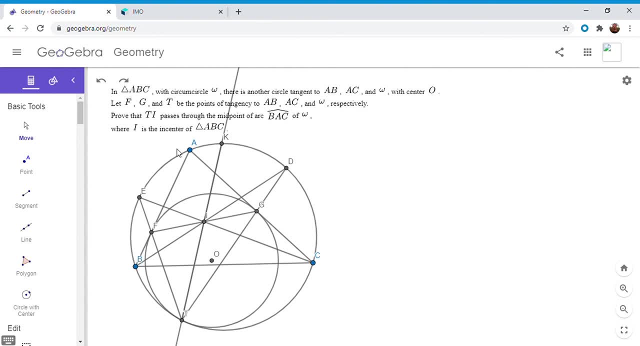 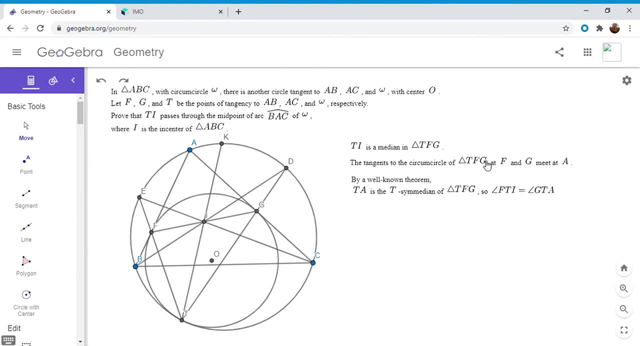 So by that theorem T A is the median of triangle T F G. So by that theorem T A is the median of triangle T F G. So because the tangents to the circumcircle of that triangle don't meet at a, T A is the simedian. 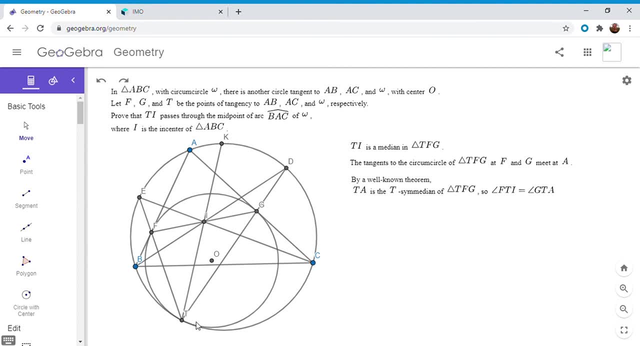 So it's symmetric to T K with respect to the angle bisector of T F, G, And so, due to that symmetry, since they're both reflections over the angle bisector, we have to have angle F. T I is equal to angle G T A. 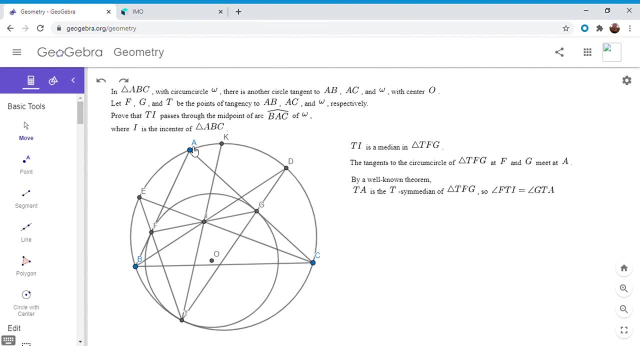 All right. So what do we do from here? Well, angle GTA is equal to angle DTA, So I'm going to do a little angle chase here. So we have: FTI is equal to GTA, GTA is equal to DTA and DTA is equal to DBA. 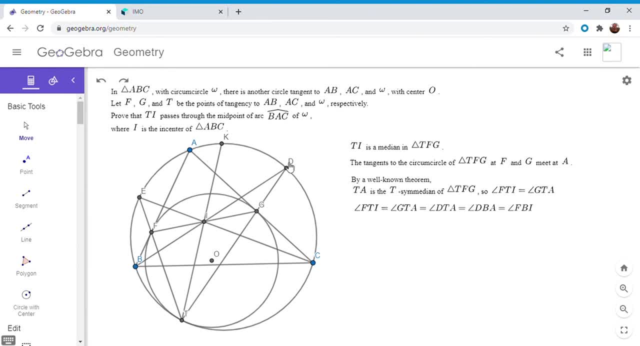 and DBA is equal to FBI. So we've shown that angle FTI is equal to angle FBI. so if angle FTI is equal to angle FBI, then that means quadrilateral FBTI has to be cyclic. Okay, so that's kind of interesting. that's another cool property of this configuration. 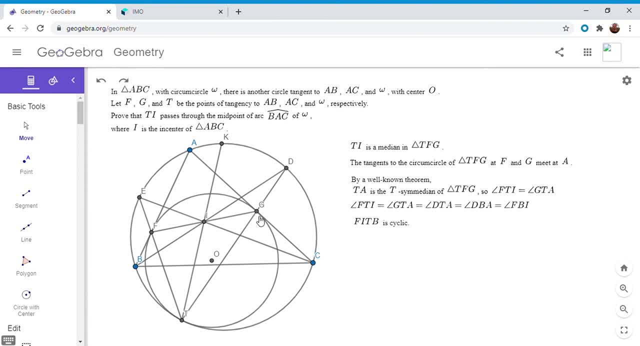 And that's then, by the same logic, GITC would have to be cyclic, So we have two cyclic quadrilaterals here. So how do we leverage that? So, ultimately, we wanted to show that K is the midpoint of arc BAC, And so that would be the same as showing that angle BTK is equal to angle CTK.